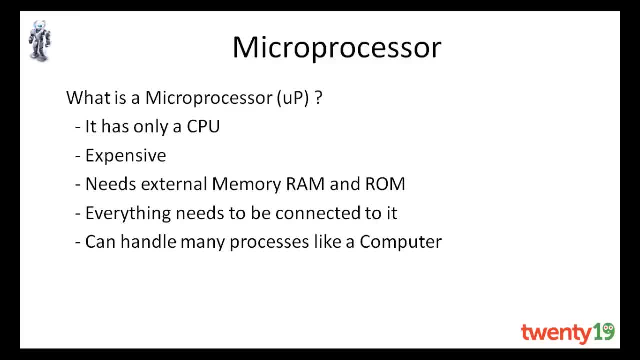 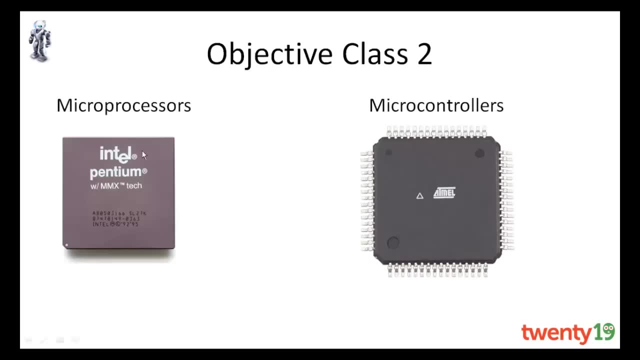 It contains only the ALU Arithmetic Logic Unit and some registers. Now, these registers are like your variables that you use to store data. Okay, Now the CPU is on chip. Now, what do you mean by on chip? Over here, this is called a chip. Similarly, this is also called as a chip. 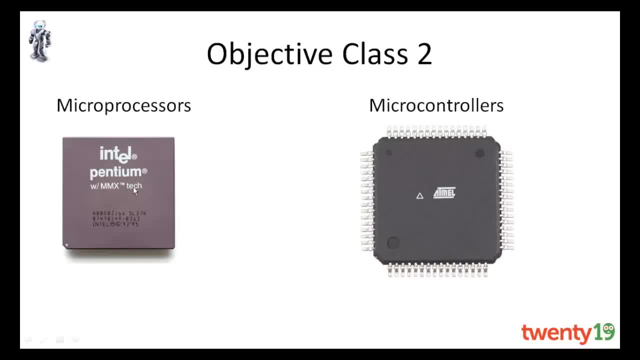 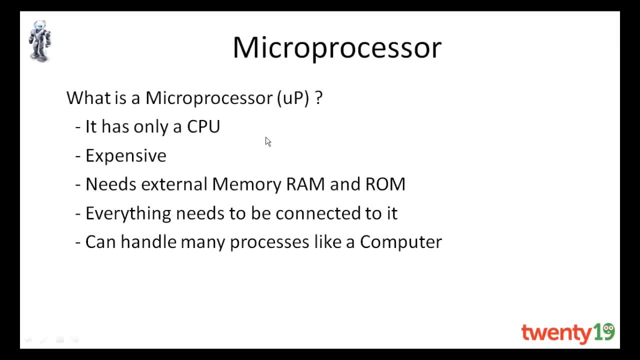 Now, on chip means it is inside the chip, It is present inside the chip. Okay, So in microprocessor the CPU is on chip. Now, compared to a microcontroller, it is expensive, Okay. Example for a microprocessor: Pentium 1,, 2,, 3,, 4, Intel Core 2 Duo, These all are called processors. Okay, 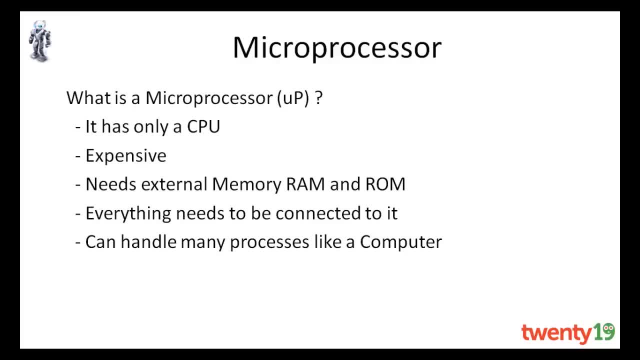 So, because of, like, they are very high-end processors. Now these processors cost around more than 30,000.. So if, as a college student, if I want to work on something, let's say I want to develop a device. 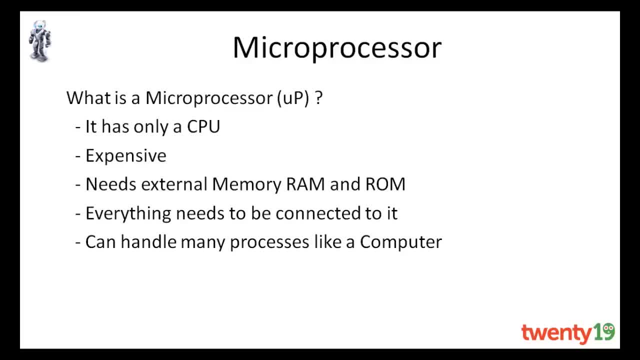 Let's say I want to develop a washing machine, So if I use a processor, the processor itself will cost 30,000 rupees, So it is not feasible to use a microprocessor. Okay, So even as a consumer, I won't like to spend 30,000 for just washing my clothes. 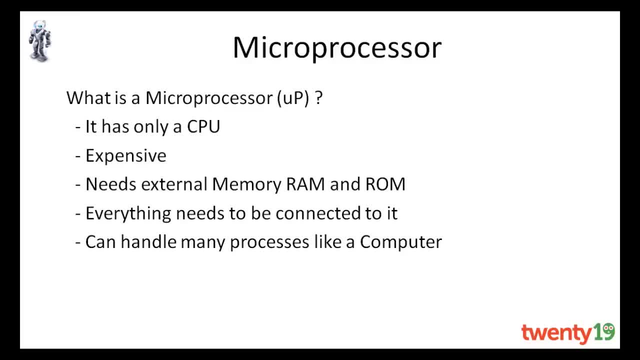 That also. that is a minimum cost just for the processor. So including everything, the motor and all, it may go up to 60,000-70,000.. Then on the microprocessor, the RAM and ROM have to be connected externally. 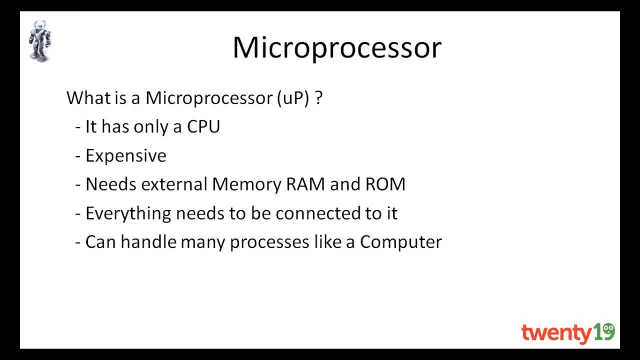 That is not present on chip. Now, RAM and ROM, like in your computers. Your computer has a RAM memory right The two slots in the computer. I hope everyone knows that In the motherboard there are two slots. You have to put a RAM memory inside there. What is the ROM memory? 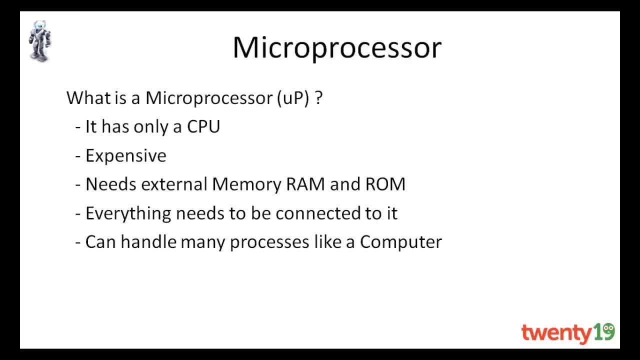 Your hard disk. Your hard disk actually is a ROM memory, So you can see, right, They both are external, They both are not present on chip. Okay, Everything has to be connected to it. Now let's say what else comes in everything. 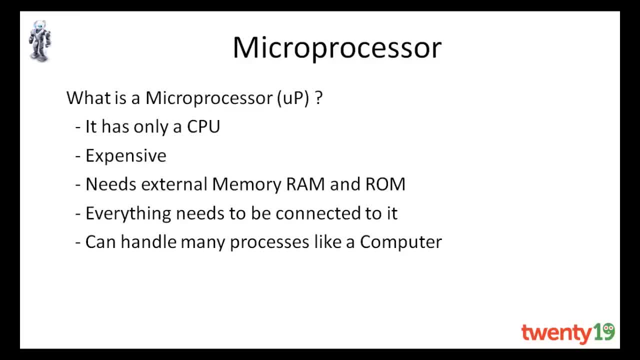 The IO port. What is the IO port? IO port, input output port. Now, in the microprocessors, the pins are just open, So you don't know what port it is. So to decipher what port it is, we use IO ports. Okay. 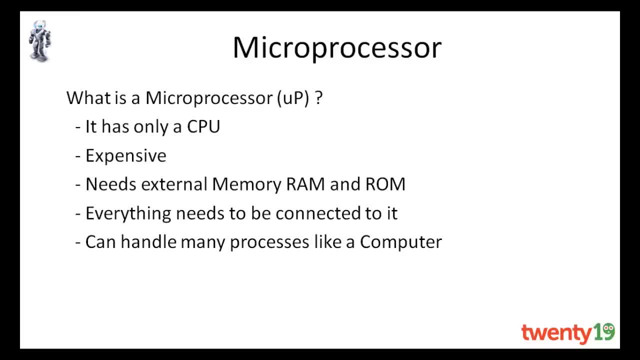 Now, microprocessor actually only processes the data, Okay. It cannot control your device. It only processes the data, Okay So, and a microprocessor can handle many processes Like a computer can- Okay, So this is about microprocessor. 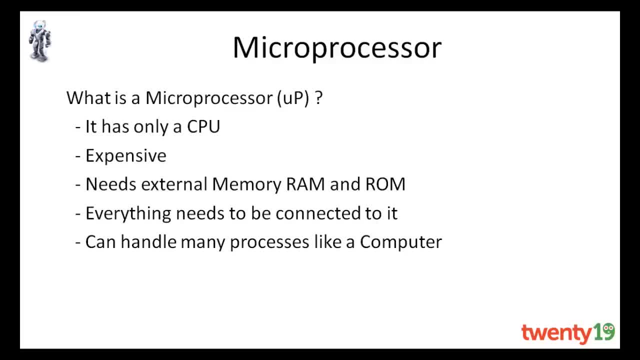 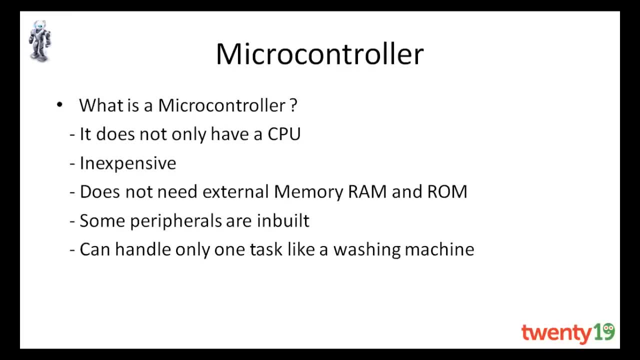 I hope you all have got a rough idea what a microprocessor is. Now let's see what is a microcontroller. A microcontroller actually does not only have a CPU. Okay, On chip, Now on chip, it has many things. 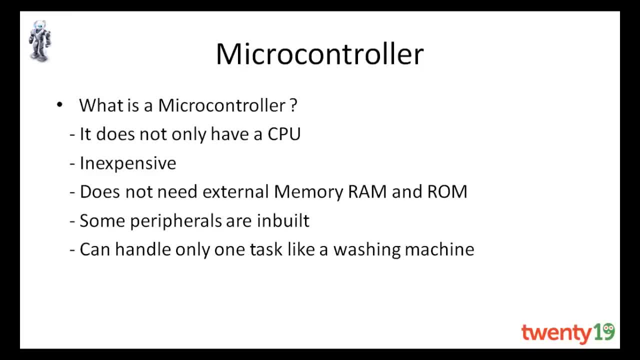 It also has a RAM. It also has a ROM And some inbuilt features. For example, some inbuilt features: ADC, Analog to Digital Converters. Okay Now, analog to digital converter is actually a hardware present on chip, So that is inside the microcontroller itself. 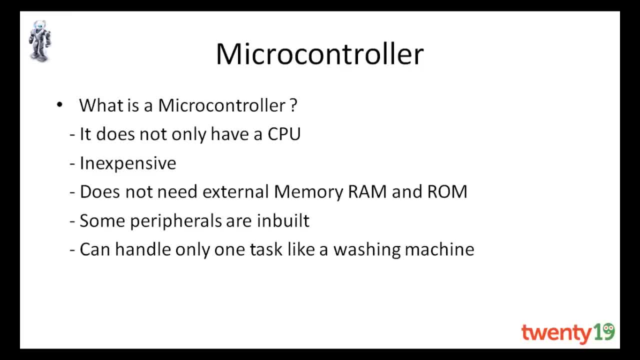 Now let's say one more thing, One more feature of a microcontroller. Let's say serial communication. Now, serial communication is used to communicate between two microcontrollers. So even that is present on chip. Okay, Now, compared to microprocessor, 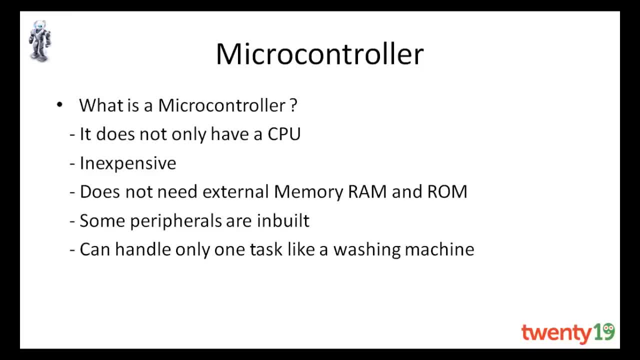 it is very less expensive. Like it may start from few, like hundred of rupees and go to thousands of rupees, So it is very cheap compared to a microprocessor. Now, controller can handle only one task at a time. 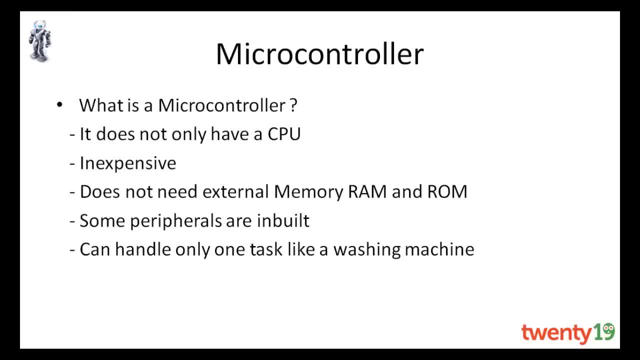 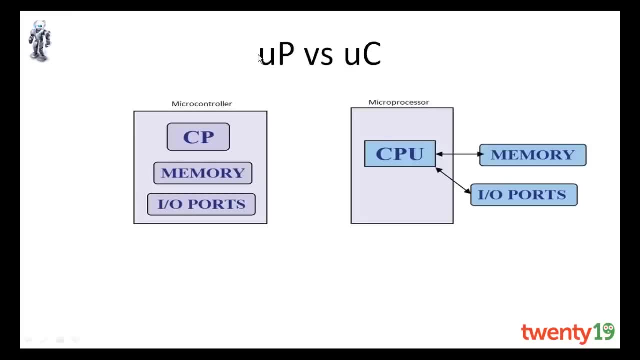 It actually controls your whole device. Let's say, a washing machine is a device, It will control the whole washing machine. We will see in the example, in the coming example. Now in microprocessor. you can see over here The memory and the CPU is in the microcontroller. 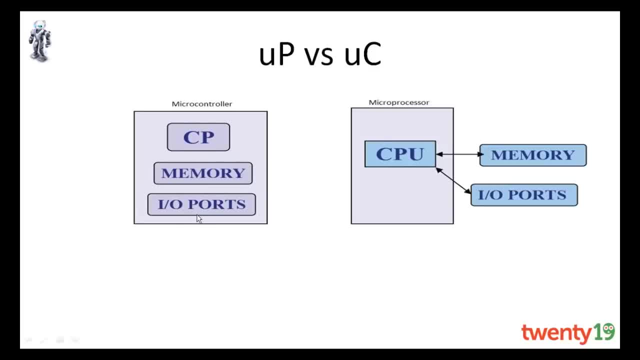 Sorry. in the microcontroller the CPU and the memory and IOPorts are on chip, Whereas in a microprocessor the CPU is only present on chip, Whereas memory and IOPorts are off chip. You have to connect them externally to the microprocessor. 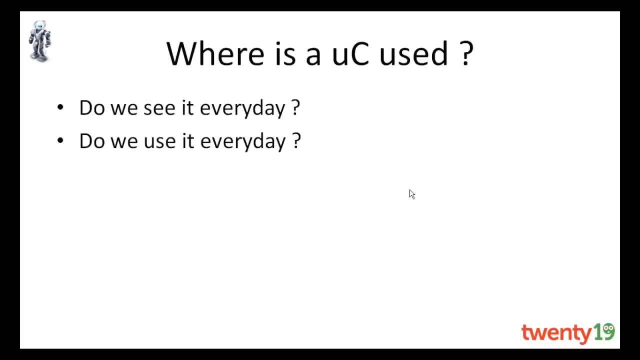 Now, where is microcontroller used? Where is microcontroller used every day? And yeah, sorry, where do we see it every day and where do we use it every day? We actually don't see it, okay, But yeah, we use it every day probably. 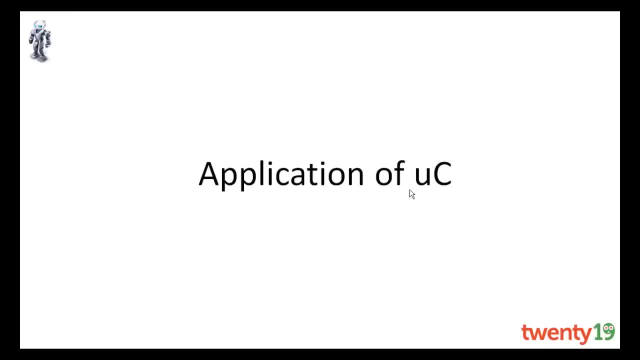 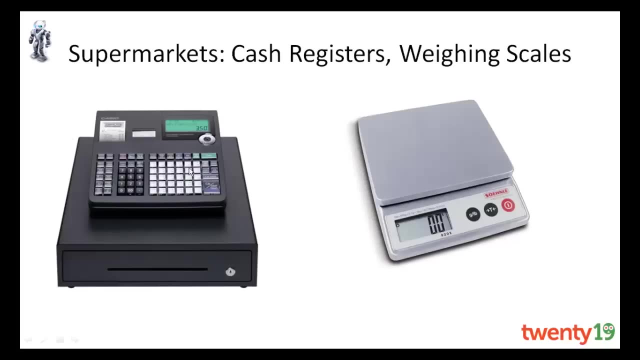 Let's see some of the examples. applications of microcontroller. MuC stands for UC, stands for MuC, Mu, micro C controller. Now in supermarkets, right In supermarkets, we have some cash registers like these. Now, using these buttons, we give the input to a microcontroller. 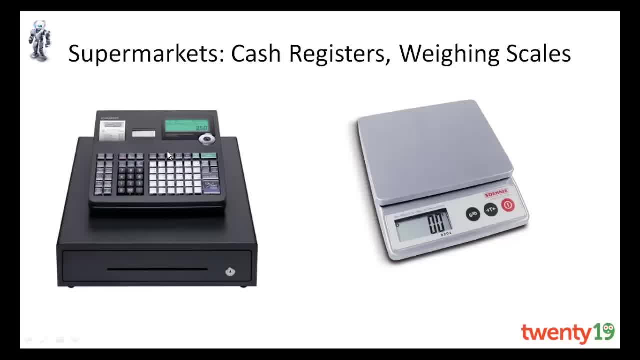 The microcontroller might be present somewhere inside over here, okay, So that microcontroller will process the data, okay, And then control it and give the data to the LCD And also print the bill, okay, So all this work is done by who? 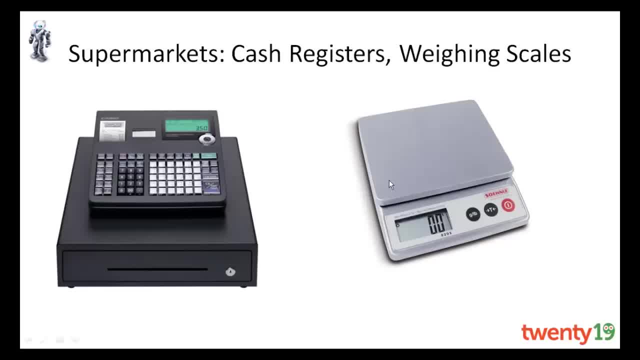 The microcontroller. Then let's say, A weighing machine. Okay, A weighing machine. you keep some, let's say, a few grams of potato on it. It will tell you how many grams it is, depending upon how much of potato you've put on it. okay, 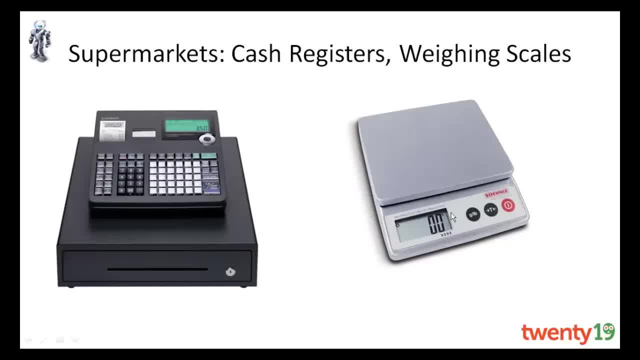 So even in this, the microcontroller will decipher what kind of weight on how much is the weight of the particular item that you've kept over here. okay, So these things are controlled by microcontrollers. These are just few examples. 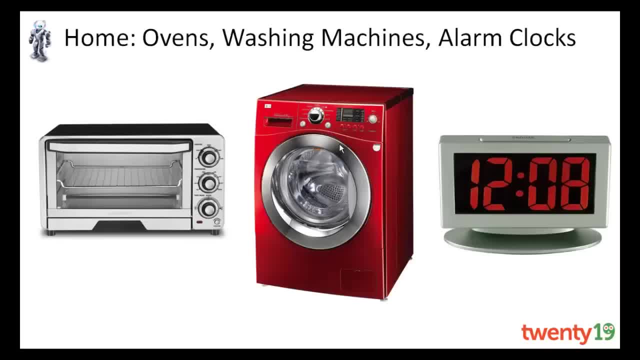 There are many of these, Then at homes, Now at homes. we all have seen an oven. Now this oven actually just heats the food, right? So a microcontroller is dedicated to do only one thing: It will only heat the food. 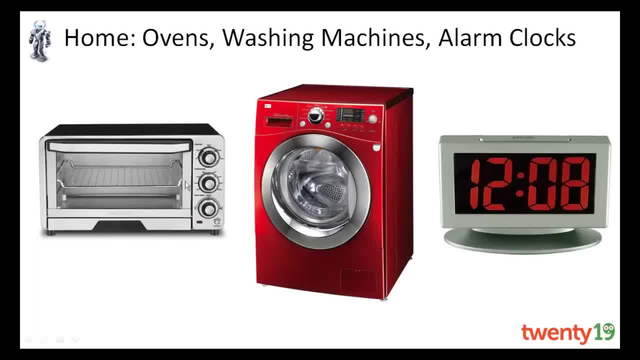 It will not wash the food, right? Yeah, So it only heats the food. Even this whole thing is controlled by a microcontroller. Let's say, a washing machine over here. Even in this, Even in this, it is being controlled by a microcontroller somewhere inside. 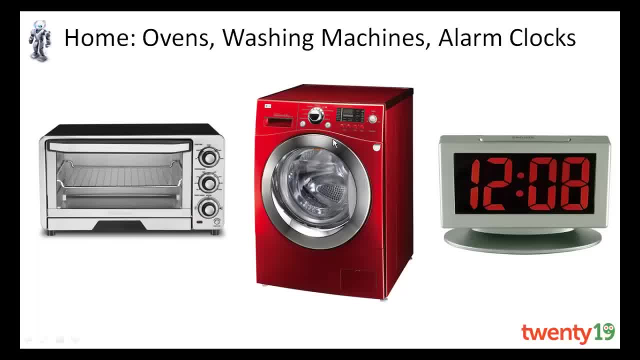 You give the data, what kind of clothes they are, how many minutes you want to wash it, put some detergent and it will wash the clothes and give it back. Then I hope everyone knows what is a digital alarm clock So I won't be elaborating on that too much.